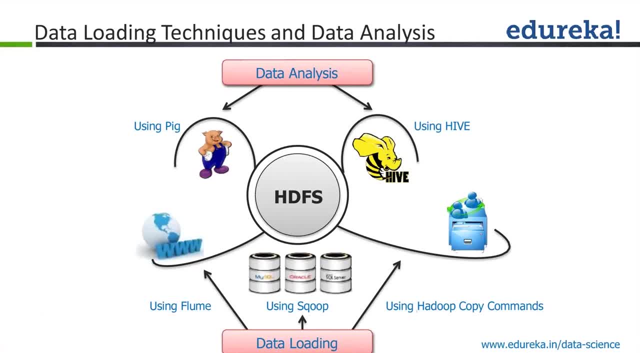 How do you load data into Hadoop system? We talked about Scoop, which essentially help you interact with relational systems like MySQL, Oracle, SQL Server and other things. You can import and export data from these relational systems using Scoop. Okay, And using Flume, you can connect to more streaming internet data sources, like Twitter, Facebook or the click stream from produced from your web server, and so on. Okay, And apart from these two, there are also Hadoop distributed copy commands, which help you transfer data between multiple Hadoop clusters. Okay. 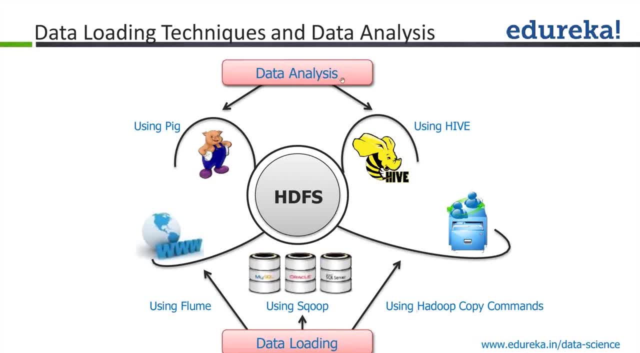 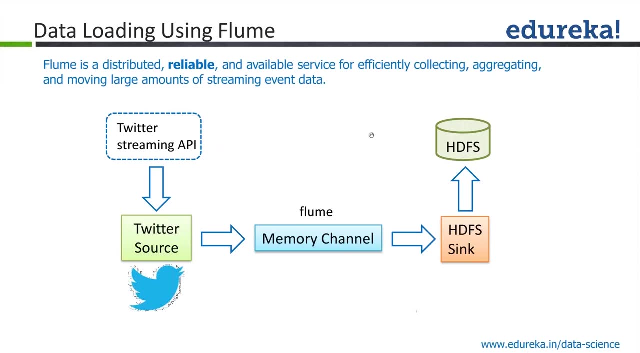 And then, once you have the data into your HDFS, you run these components like Pig and Hive to do some data preprocessing and data manipulations. Okay, This is something you will see in one of the LMS sections which help you kind of: help you install Flume, help you install Hadoop and let you connect to a Twitter streaming API and get the data, store it in HDFS and do some processing on it. 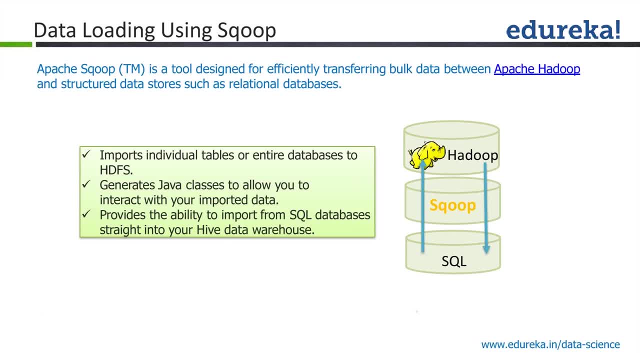 Okay, What's the one big challenge that Hadoop is not able to handle when compared to RDBMS? Transaction semantics. Hadoop doesn't have transaction semantics, Whereas RDBMS thrive on transaction semantics. right, Whenever I withdraw money, whenever I deposit some money into my bank account, I need strict transaction semantics, Otherwise I'm not going to trust RDBMS. 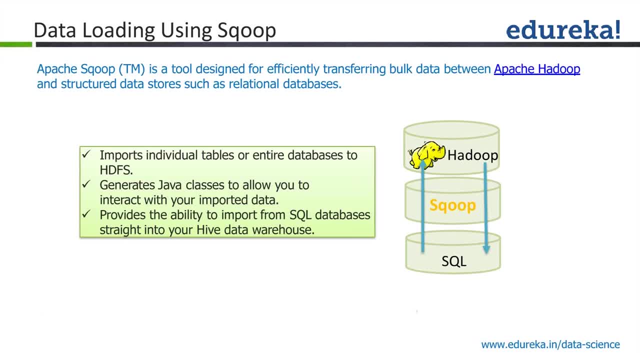 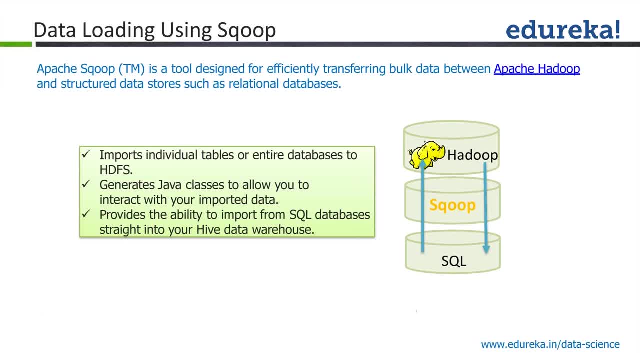 the first class about schema on read and schema on write right. which kind of place an important role in the sense that in case of our DBMS, you need to have the schema ahead of time before you start putting any data into the system, whereas in Hadoop you dump everything that you have. okay, it's up to the. 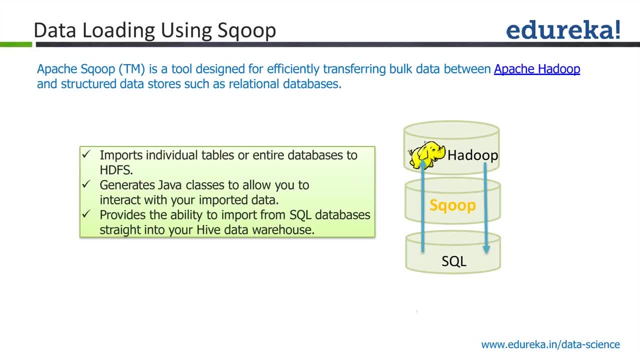 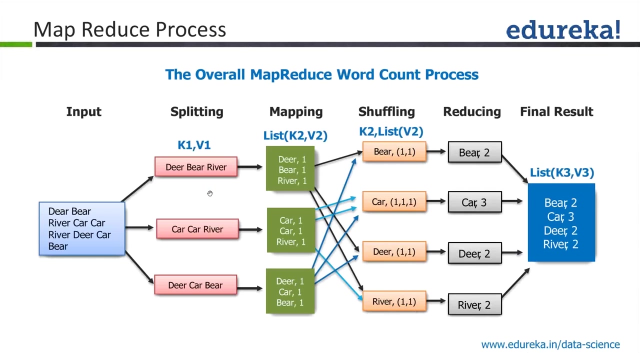 application, with whatever is using the data, will read the data in appropriate format through this concept of input formats. okay, so you define the schema on read, not on write. okay, that's another key, very, very important distinguishing aspect between the two systems. okay, so this is what we want to talk about. okay, so this slide covers essentially the 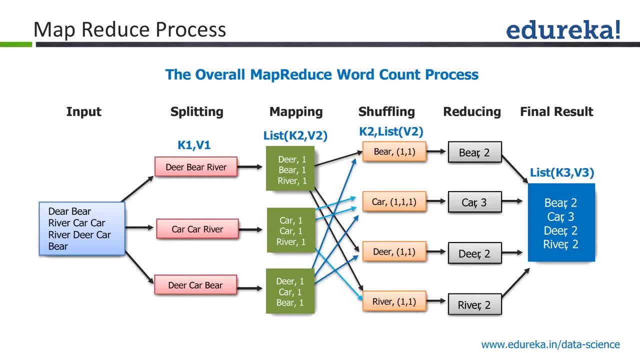 aspects that we need to know about MapReduce programming paradigm. right, as, as we told, MapReduce consists of mappers and reducers, right, so those are the key processing engines in the MapReduce job. okay, and let's see how does a MapReduce job runs. so now, basically, this MapReduce job should take some input, does some processing and 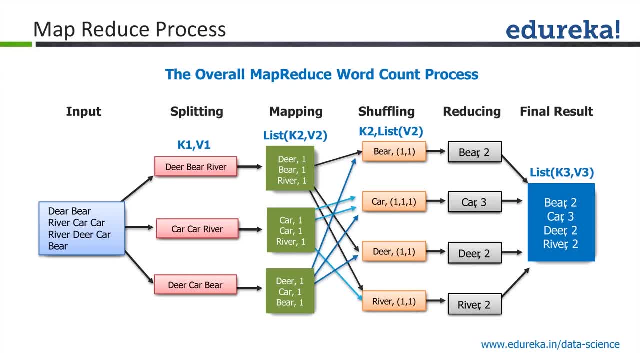 produce some output. okay, so this is like a HelloWorld example of MapReduce, which is a word count. you have an input data file and you want to count the occurrences of a number of occurrences for each of the word, and the output that you produce is something like this: okay, so the input data set is this and the 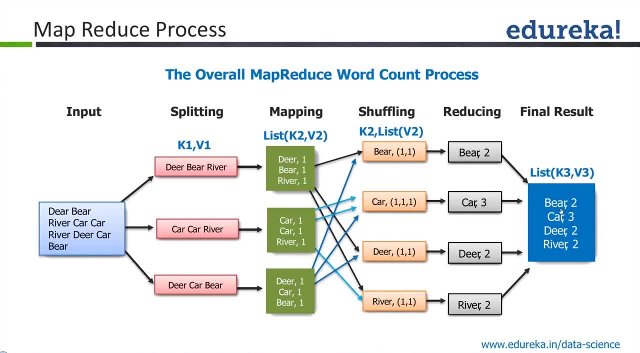 output data that you produce is something like that. this output data set is this, which is simply the number of occurrences of each of my word. okay, and I want to do this in a parallel manner using MapReduce functionality. okay, so the first thing, what did we say? whenever a client submits a job, we will go get. 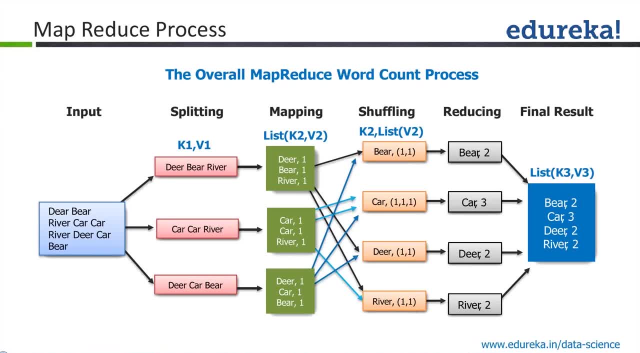 all the metadata about the file regarding the number of blocks, number of the size of the input and everything, and then we logically split this data set into- logically partition data set into splits. okay, so, though, these are the splits that you get. okay, so, from this data set, we split it up into individual. 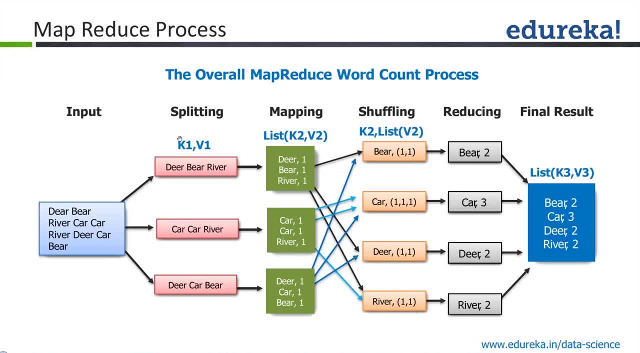 splits and in each of the split your data is represented in the form of a key value pair. okay, there is a key aspect and there is a value aspect and there are many input formats which kind of tell you how to define this key and value. my simplest format is called as: 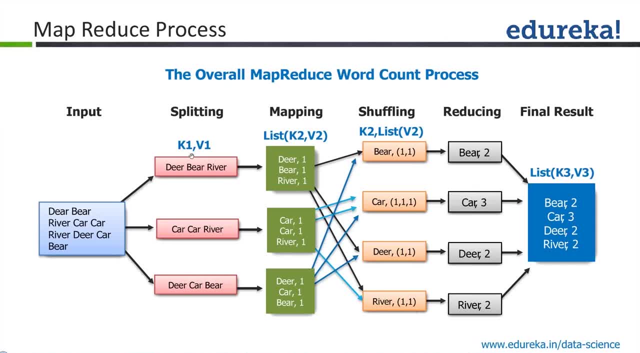 text input format. that means I am just reading my data line by line. okay, so the key will be like a position in your file and the value will be the entire line, entire text line that you read from your file. okay so, but the point that you need 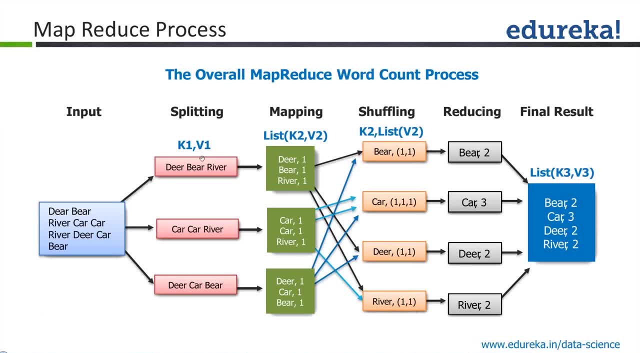 to know is, by controlling the input format, you define how to read your data. okay, this is what I mean by schema. on read, you are defining the key and value, which is how you want to read the data: at the time of reading, not at the time of writing, unlike database systems. okay, so by 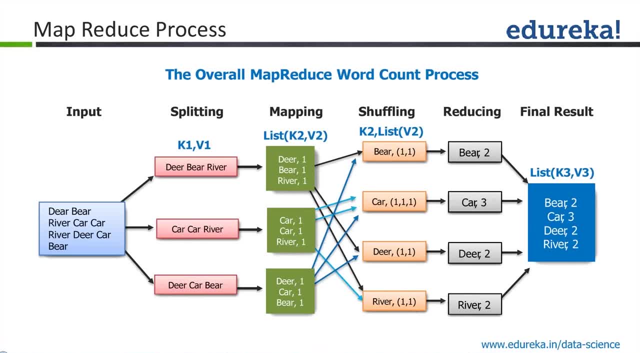 So once you logically partition your data into these splits and your data is organized as key value pairs, as governed by input formats, on each of this input split you apply your map function. So this is a map function that you implement using your mapper process in Java. 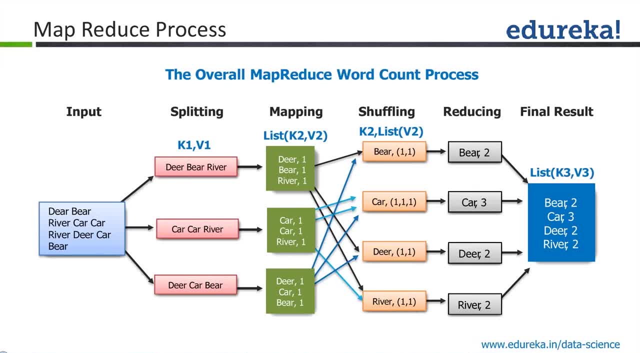 The way you implement that process is: you assume that you get a key value pair from your input and this mapper function will tell you how to process that key value pair and then produce another list of key value pairs. So that means it consumes a key value pair- k1, v1- and it applies the map function and 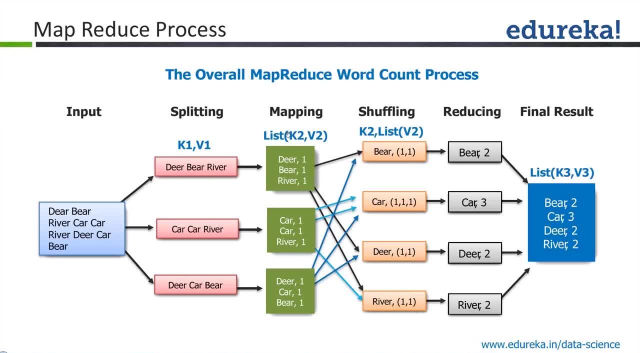 produces another list of key value pairs. So it's a list of k2, v2,. it may have a different key, different value, or it can be the same. it doesn't matter. The mapper function will decide what this k2, v2 will be and how this k2, v2 are computed. 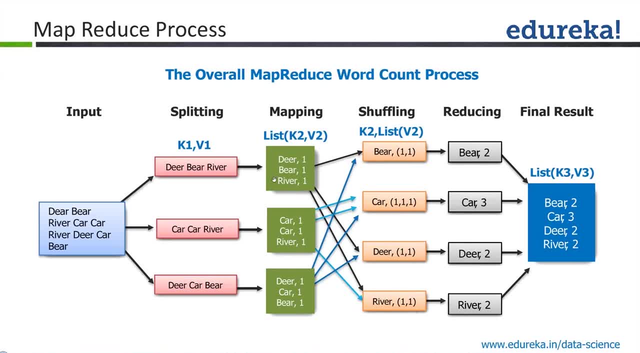 from my k1, v1.. That's the definition of mapper function. It takes a key value pair of the input, it does some processing and produces a list of key value pairs. Okay, And in this particular case the word count example. so the way the mapper can work is: 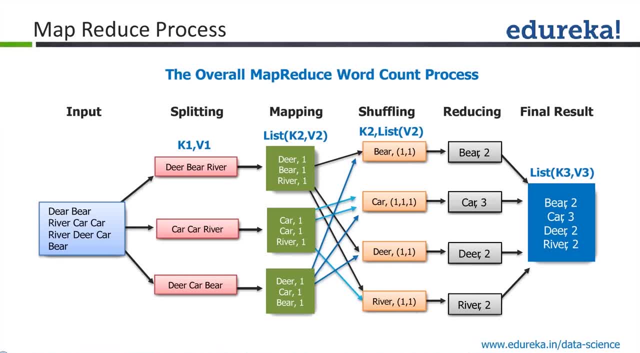 essentially, it reads a line, it splits the line into individual words: okay, And for each of the word I'm going to output a count called one okay, Because that's the word that I've seen once. So I read these three words as a single line. 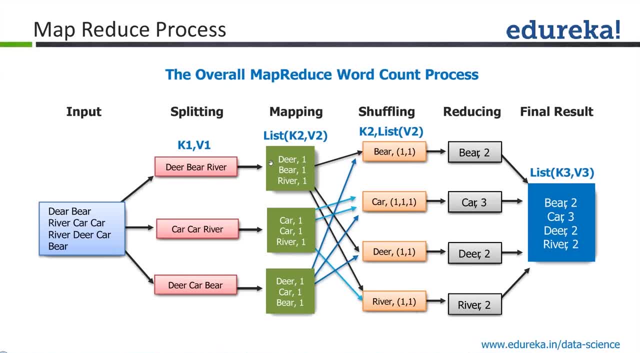 D r v, Bear and river, And so this mapper function or mapper task to be precise. this mapper task reads this: k1, v1.. Okay, K1 is some offset index in my file and v1 is this entire line. 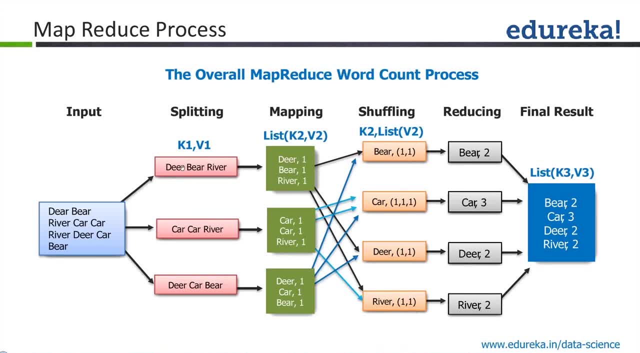 And the mapper function tells you that. okay, I'm going to read this data. I split this line into individual words- D, r, v, Bear and river- And I'm going to output the counts, one one, one for each of this word. 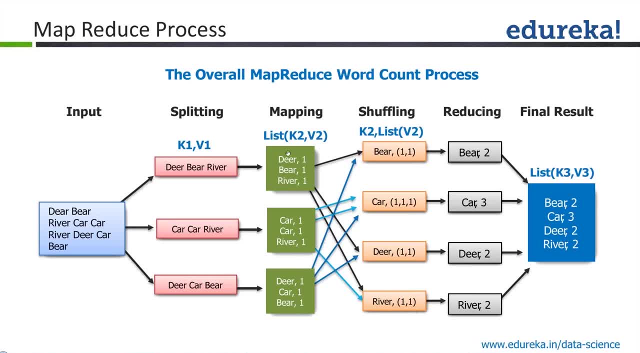 Okay, So my list of key value pairs will be this: My key is a string consists of a word and my value is an integer. okay So, and similarly, the same thing will be done on a different map task as well. 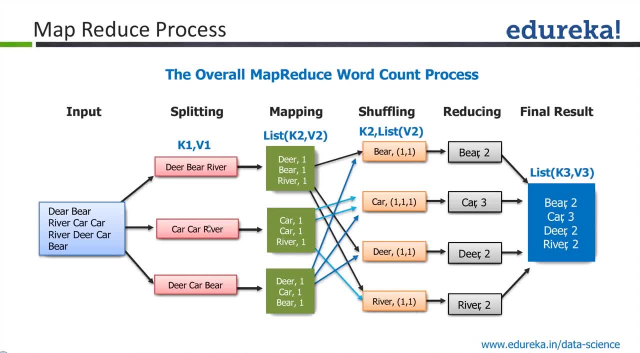 So the different map task will read: a different input split consists of a different input line: K1, v1.. Okay, And then in this case, k, k, river, And I'm dividing that into individual words, splitting that line into words, and then I'm 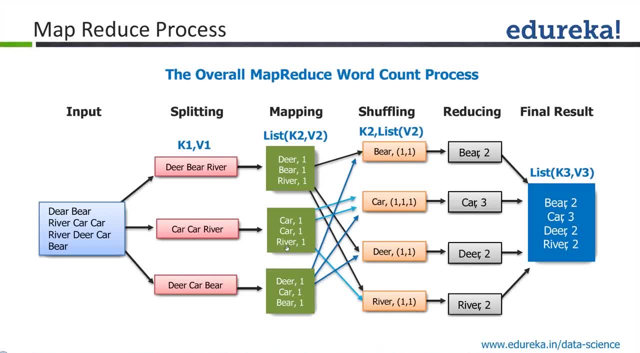 outputting counts one for each of this word. So the key value pairs that are produced by this mappers will be these key value pairs. Key is the word, value is the count of one. Okay, And similarly, the same thing is done by the third task. 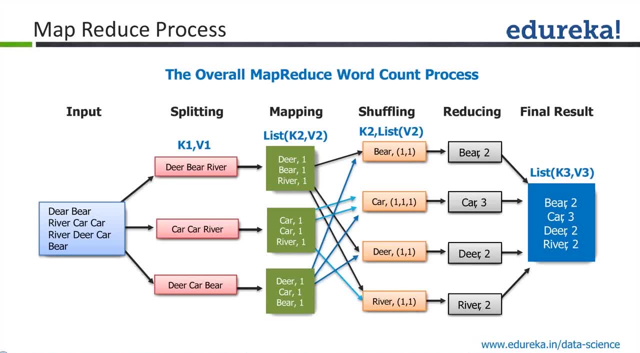 Okay, So the key thing that you can observe here is the core functionality of the map. The core functionality is exactly the same across all the map tasks. It's just that that functionality is applied on a different portion of the data. Okay, And that's why each of this can run on a different machine in parallel simultaneously. 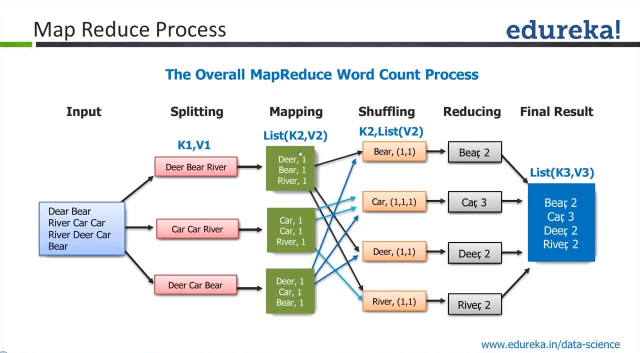 Okay, Now the list of key value pairs produced by each mapper are then passed through something called as a shuffle phase. Okay, Okay. So yeah, our mappers are essentially outputting this list of key value pairs, And in the shuffling phase it's pretty simple. 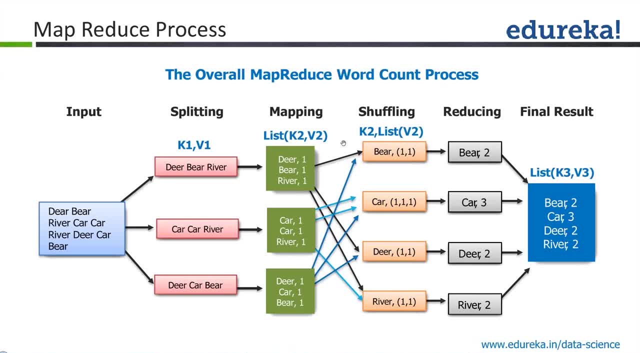 You simply sort by the key. Okay, That means you want to bring all the values For a given key together into one place. Okay, So I have dir produced by mapper one and dir produced by mapper three. Okay, Since they both have the same key, I want to bring both of them together into one place. 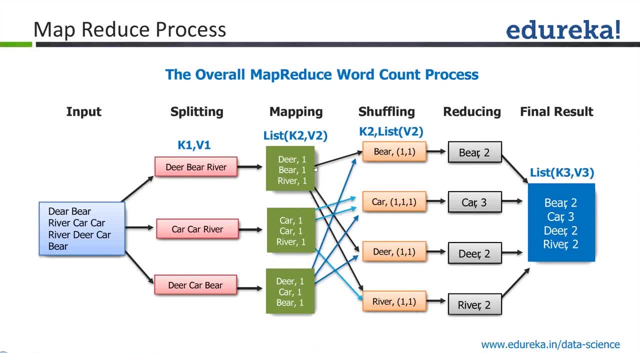 And say, a single key dir and has multiple values, One produced here and one produced here, So one come upon. Okay, So that's it. So that's it, So that's it. So, essentially, you're converting this list of key value pairs into key comma list of values. 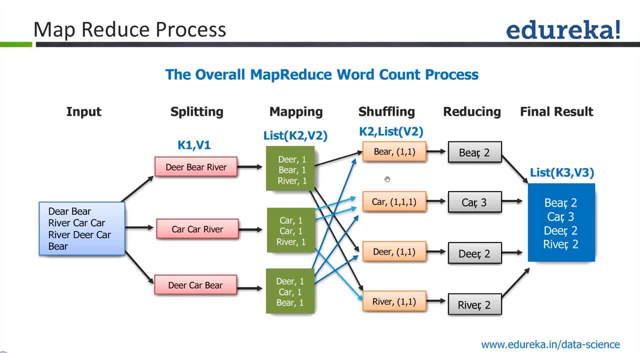 Okay, It's pretty straightforward. So you do that sorting And then you get all the values associated to bear in one place, All the values associated to car in one place, Dir river, and so on. Okay, And your reducer functionality will simply tell you how to reduce this list of key value. 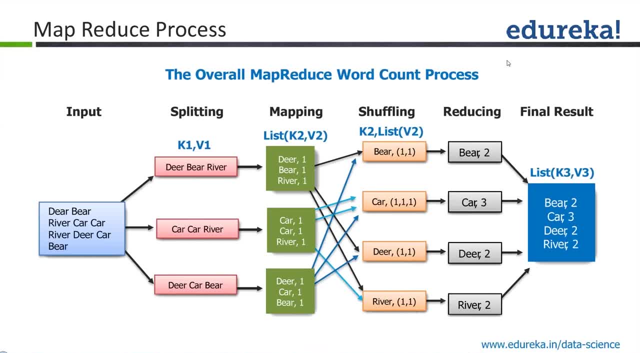 And that's why it's called reduce, because you're reducing the list of values associated with single key into another list of key value pairs. Okay, And in case of word count, it's simply adding up all these numbers. Okay, I add one plus one. 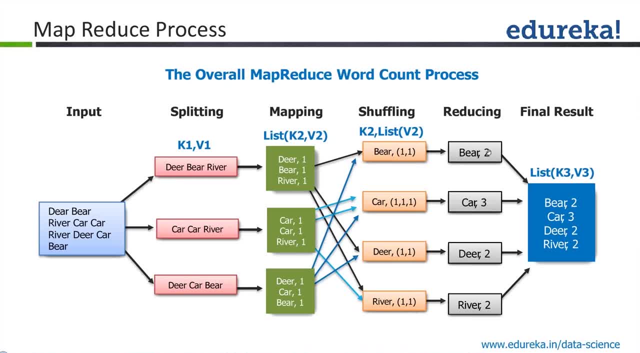 So I get the same key bear and the count two. This is what I output from my reducer, And in this case I am adding up all the three, So I get car comma three. Okay, So that's essentially a MapReduce job. 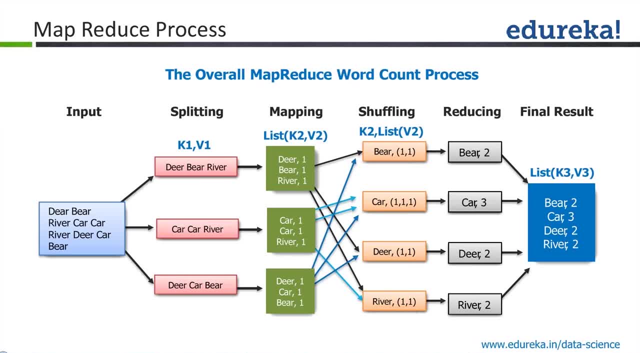 You are starting with an input file, You are splitting into some logical splits And you read this: data set data splits as key value pairs And then each mapper will consume key value pair and produce a list of other key value pairs, which can be same or different. 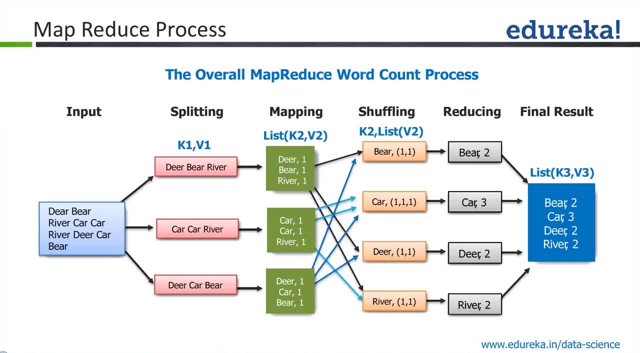 Okay, Okay. And then in the shuffling you bring all the values corresponding to a single key together in one place And then reduce functionality, will reduce the list of values associated with this particular key and then produce another set of list of key value pairs, which will be the final output of your MapReduce job. 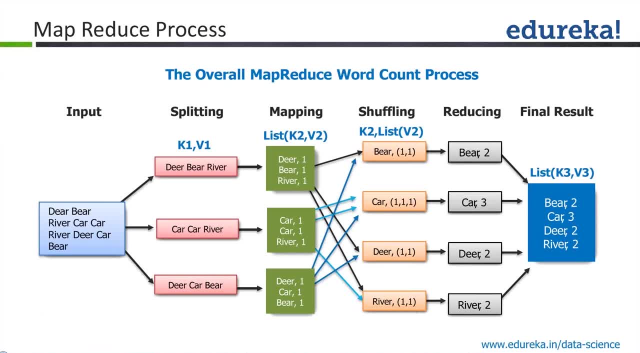 Okay, Now if you are in your MapReduce world and if you want to do something, let's say I just gave an example of Aggregation, right, or k-means clustering. So linear regression also can be done, but let's say k-means clustering. 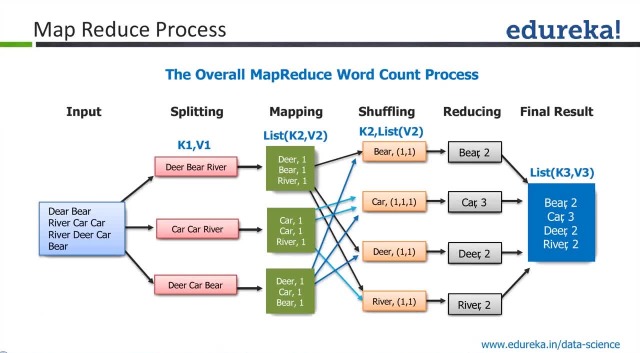 If I want to do k-means clustering in MapReduce, I have to imagine how to organize my computation into my mappers and reducers. Okay, If I want to do k-means on MapReduce, how would I do it? So what is k-means? again, 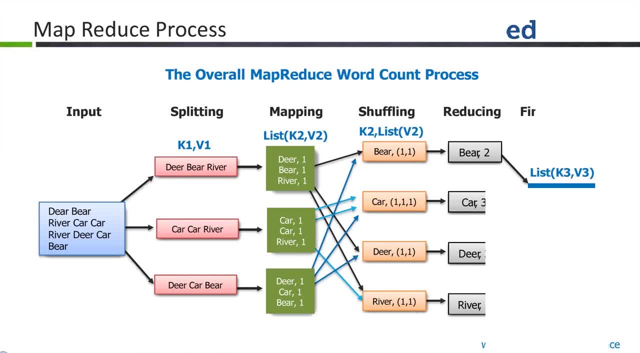 If you Okay, Remember, we have these k-cluster, k-centers and we want to compute the distances from each of my data point with all the k-centers, Right. So let's say, somehow I gave k-centers to all my mappers right in a distributed manner. 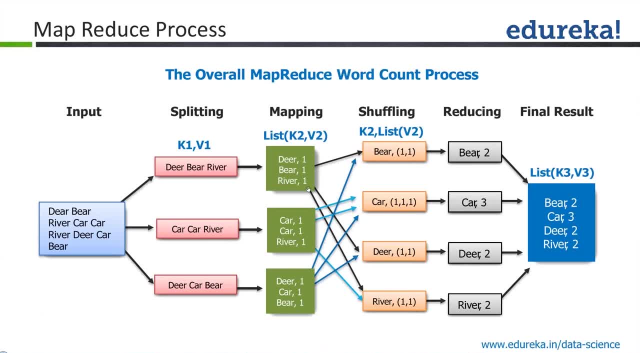 So each mapper has all the k-centers. Now each mapper will get some partition of the data. Okay, So I have the entire data. So I have the entire data set on which I want to run k-means. 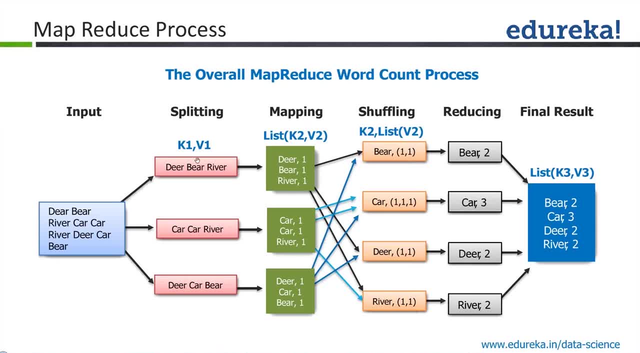 And my input formats, my logical splits, are some partitions of my data. Okay, Now each mapper and the key value pair in that sense will be key, will be like a record ID and the value will be the entire record. Okay, 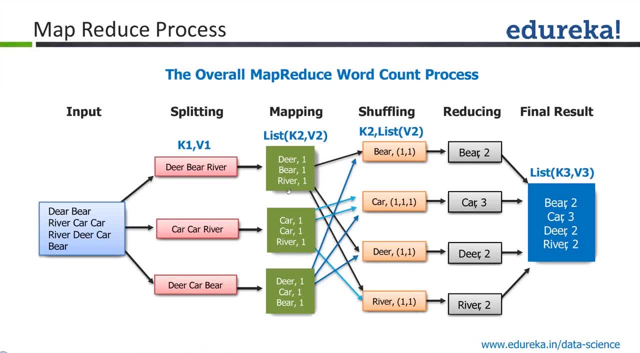 And that's controlled by my input format. Now the mapper has access to all the k-centers. Okay, Now it will read: First key value pair. that means the first record, And then it computes all the k-distances. 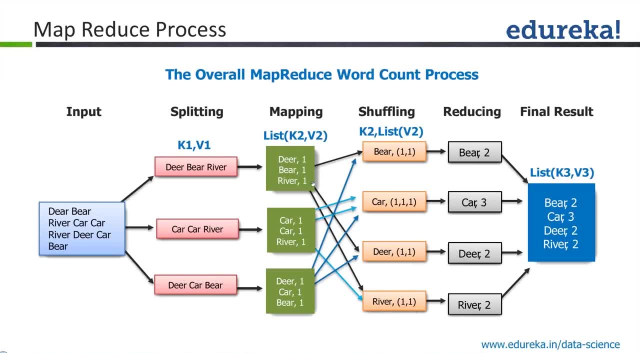 Okay, Between that value and all the k-centers, And then I can output my results, which are the distances between those k-centers, And there my key can be the center ID of the center And the value can be the distance. 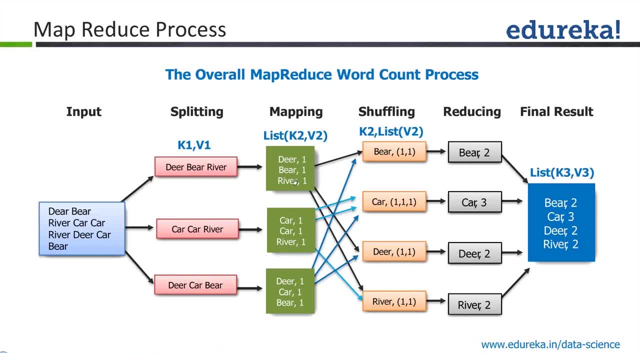 Okay, Okay, And and also probably, I need to output the data point in order to compute the new centroid And similarly, that's done by all the mappers. Okay, Now, through the shuffling, I get basically all the distances associated with the single center.